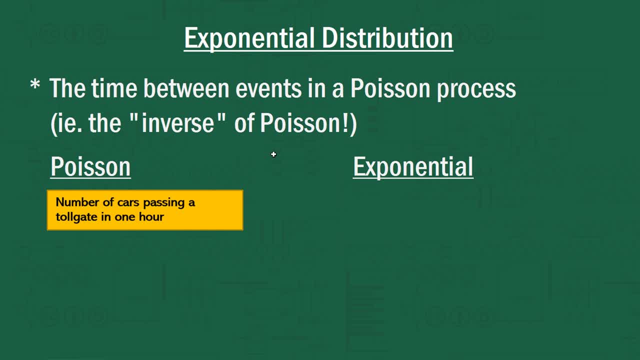 Poisson distribution might be the number of cars passing a toll gate in one hour. So that's like the classic example they always give for a Poisson distribution. To turn that into an exponential distribution, we might say it's the number of hours between car arrivals. So it's almost like 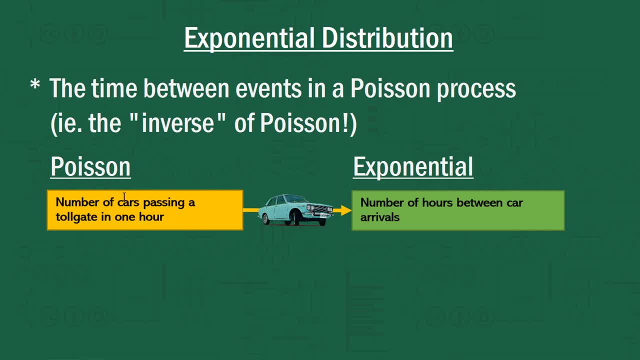 you're flipping it on its head, right. So instead of looking at cars per hour, you're kind of looking at hours per car. So that's why I was trying to say it's like the inverse of this Poisson distribution. 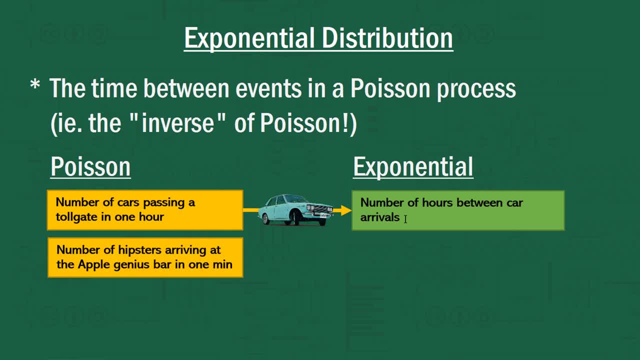 So another example might be the number of hipsters arriving at the Apple Genius Bar in one minute- And if you've watched my videos, you know I like to rag on both the Apple Corporation and hipsters. But to turn this around, we might say that the exponential distribution might be for. 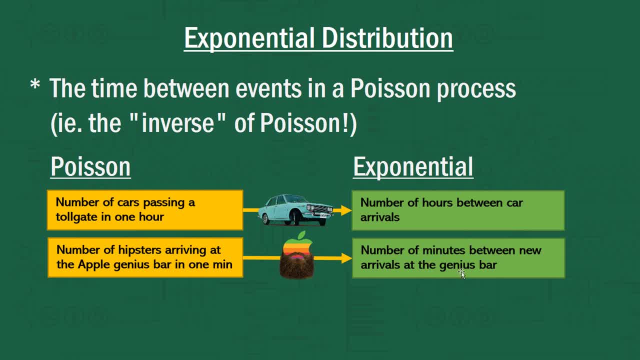 the number of minutes between new arrivals at the Genius Bar. So you can see, it's the same thing: Hipsters per minute, minutes per hipster. And finally- this is an interesting one as well- The number of soldiers killed by horse kick. So this is the number of soldiers killed by horse kick. 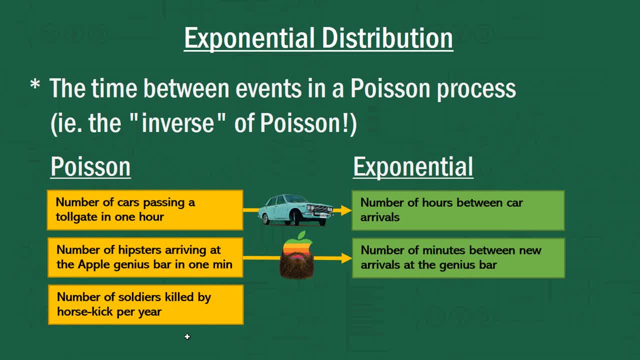 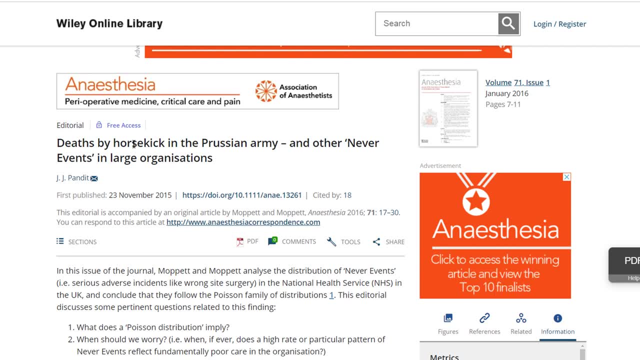 per year. Now you might be thinking: what Where does that come from? Well, interestingly enough, I'll see if I can find it for you. Let me just have a look at this. There was a very famous study done at the end of the 19th century about deaths by horse kick in the Prussian army. 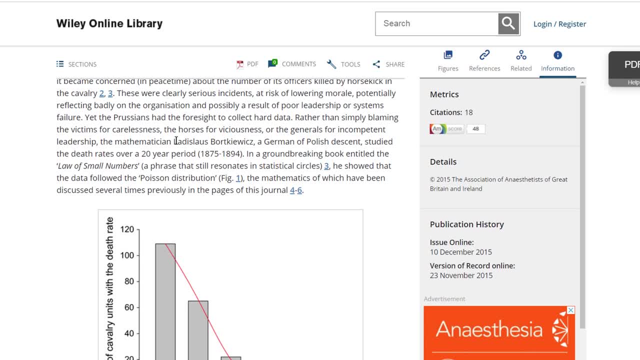 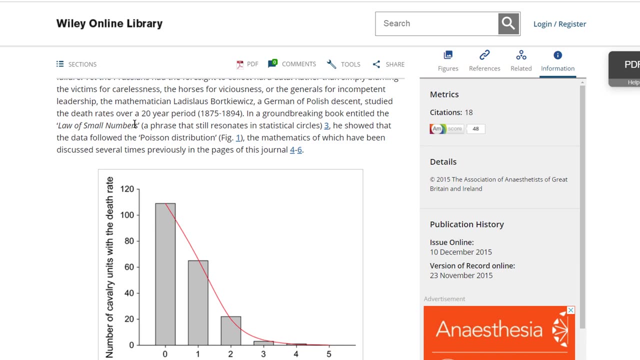 Essentially what the mathematician who ran this study did- his name was Ladislaus Bortkiewicz- basically looked at death rates over that 20-year period, 1875 to 1894. And it is horse kick deaths which are very rare events- And he wrote some book called The Law. 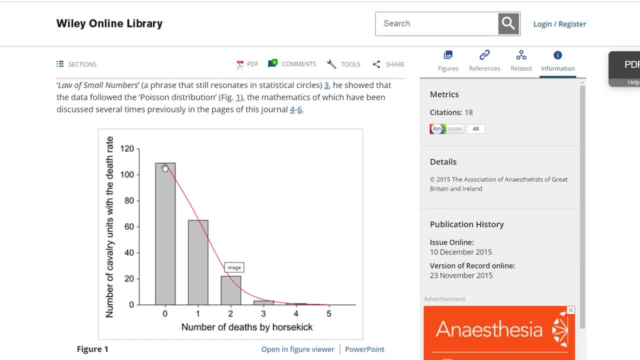 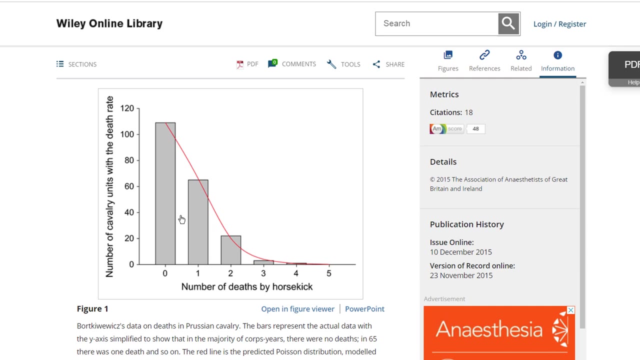 of Small Numbers. Anyway, the reason why I want to show you this is that he found out the number of deaths by horse kick per year and tallied it into this table and found guess what. It looked a little bit like a Poisson distribution. Anyway, it became like a kind of cult study, if you can. 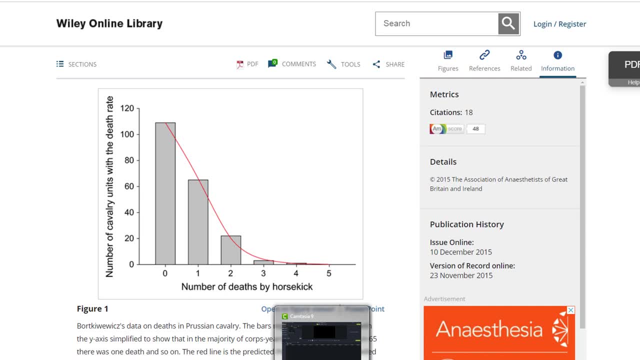 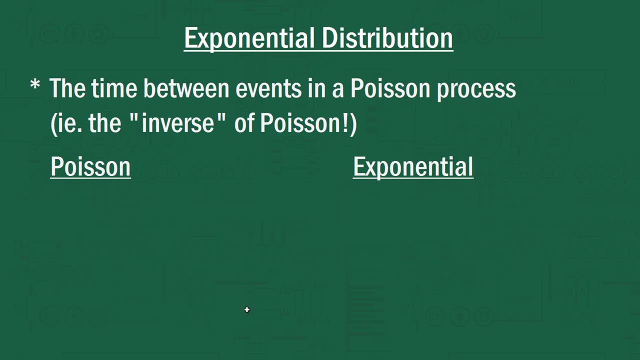 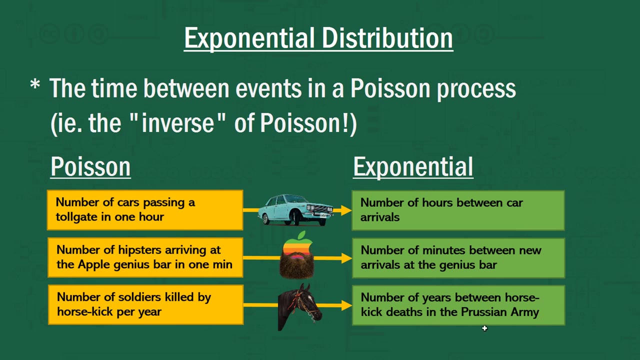 say that And it often gets referenced when we talk about the history of the Poisson distribution. But to go back to what we're talking about, if we're going to turn this into an exponential distribution, it's the number of years between horse kick deaths in the Prussian army. So if 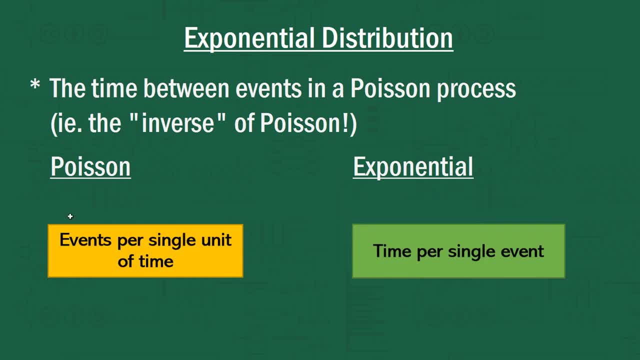 you're catching on with the theme here. the Poisson distribution might be events per single unit of time And the exponential is the time taken for a single event to occur, Or in other words, you might want to say the time between events. That's another way of looking at the exponential Same. 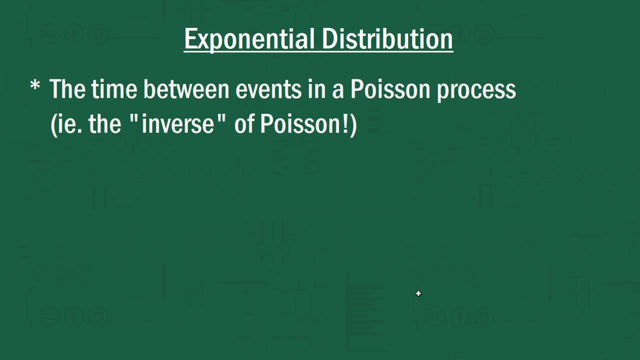 thing, just a different phrasing. Okay, so we now know the link between the two, But just in case you might want to refresh your memory about the requirements of both, the Poisson and therefore the exponential distribution, But the events must occur at a constant rate and they must be independent of each other. So if we keep 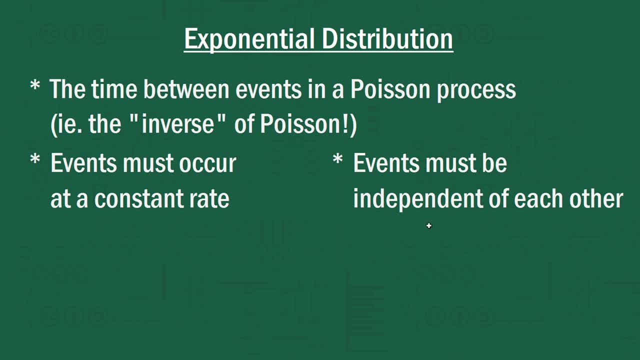 on with our horse kick example. if there were a lot of horse kick deaths in one year, the next year isn't affected by that. Now, if you combine these two requirements of the exponential distribution, we can say that the exponential distribution is memoryless, or in other words, it bears the 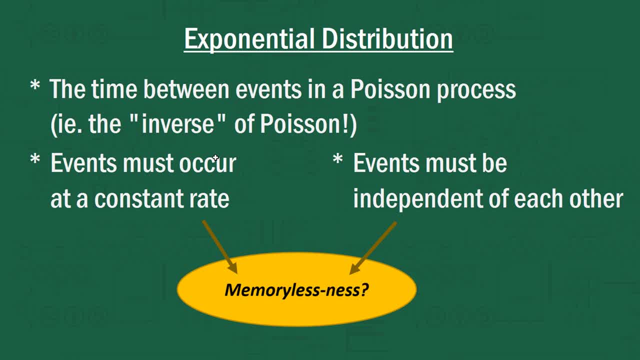 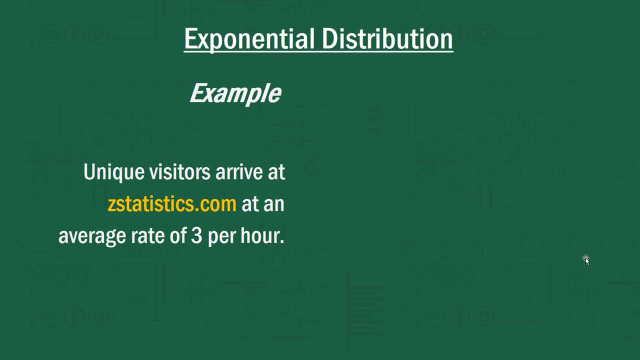 characteristic of memoryless-ness. Now, I'm going to deal with this at length at the end of this video because I don't want to get bogged down here. It's a bit more of an advanced topic about memorylessness, Okay, so let's look at the example we're going to be using for the remainder of this. 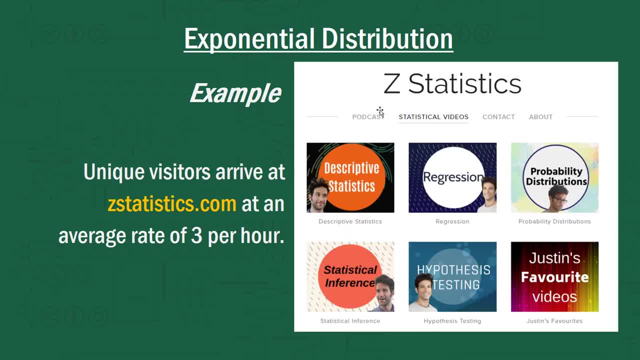 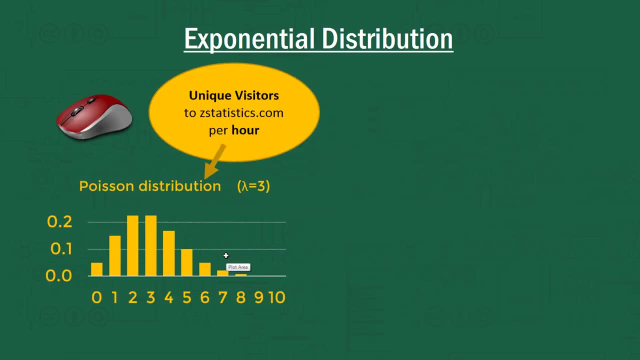 video. Let's just say that unique visitors arrive at my website. deadstatistics. there it is at an three per hour. You might realize that, yes, this in fact looks like a Poisson distribution. Well, let's see how we get to the equivalent exponential distribution. So here we might have the unique. 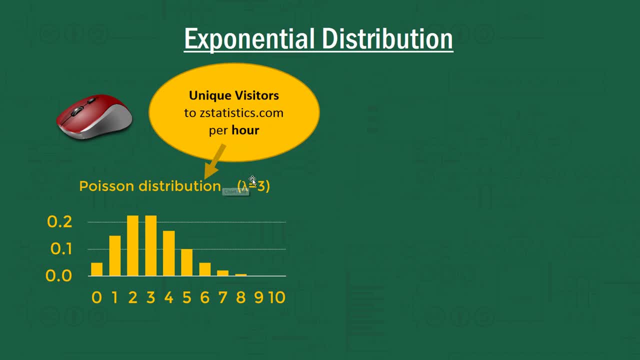 visitors to zstatisticscom per hour and we have this thing called lambda, which is the average for the Poisson distribution. Now that needs to be given to us and you can see that if the average is three, we're probably the most likely to get around three or two, maybe four, within an hour. 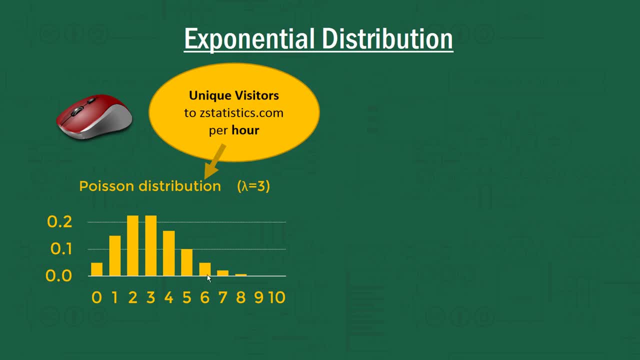 and it becomes a bit less likely to get five people per hour, even less likely to get six and seven and eight gets, and much less likely still. So this is what's called the probability distribution, or more specifically we call it the probability mass function. So I'm going to introduce to you. 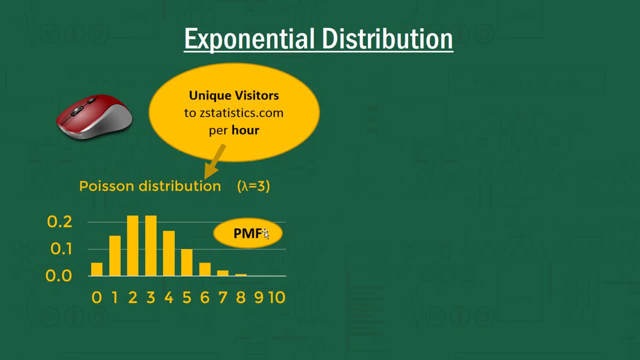 a few of these terms that you might see in your grander study of statistics. PMF, Probability Mass Function is used for a discrete distribution like the Poisson distribution is Right, you can only get discrete outcomes. We can't get two and a half people coming to my website. 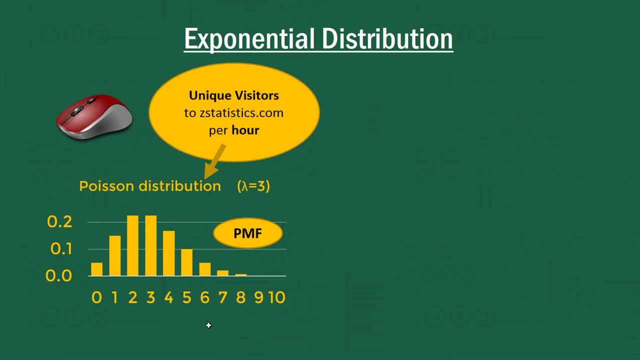 in one hour. right has to be two or three. So how do we get to the exponential distribution on this side? Well, instead of being number of visitors per hour, this is going to be the number of hours until the next visitor or next arrival at my website. So instead of the mean being three, 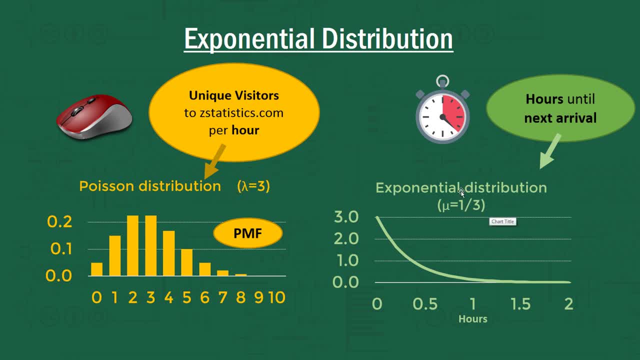 see how lambda's three over here. The mean for this exponential distribution is one on three, and we give it the letter mu as opposed to lambda. now it's not so difficult to intuit why the mean has to be one on three. i mean, if you think about it, if i'm averaging three visitors per hour, that's. 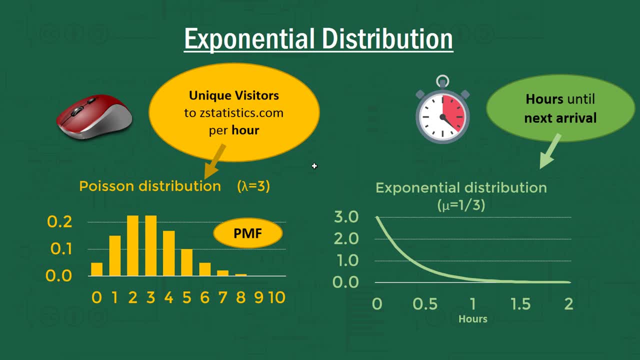 about one visitor every 20 minutes, right? in other words, one visitor every third of an hour. So that's how we relate the mean of the Poisson distribution to the mean of the Poisson distribution mean of an exponential distribution. It's actually just the straight inverse Lambda. 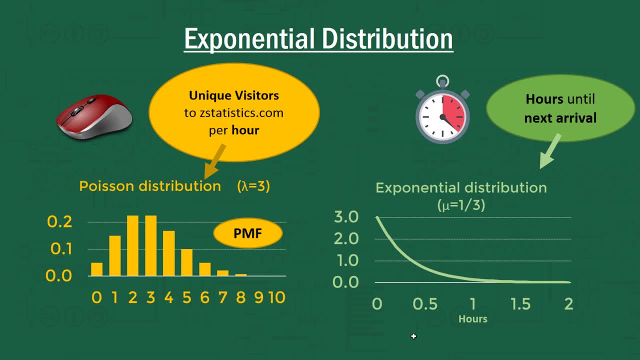 is one on mu and vice versa. Now this is called the PDF and it's the same idea as the PMF. but because the exponential distribution is a continuous distribution, we don't call it a probability mass function, we call it a probability density function. Now you might. 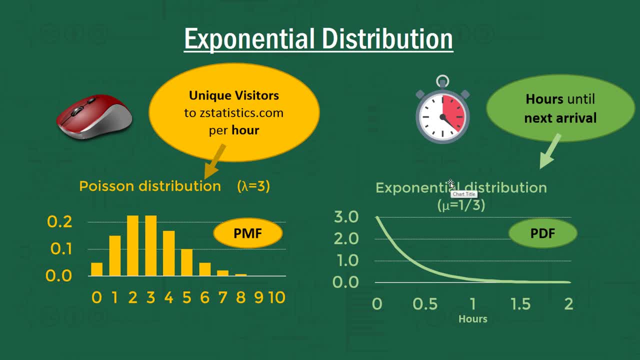 be sitting there thinking: all right, why is the exponential distribution continuous, whereas the Poisson was discrete? Well, that just depends on the units we're talking about. right, You can't have half a visitor, but you can have half an hour. In other words, 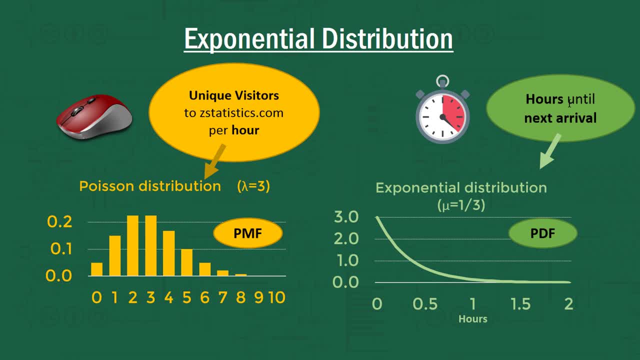 you can split up time into fractional units. So it is quite interesting that this is a nice smooth curve being the probability density function, whereas for the Poisson it's a discrete, chunky distribution which we call the probability mass function. Now another question: you might 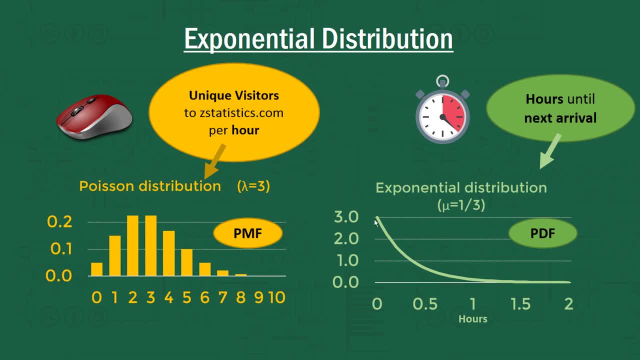 have is, why does this exponential distribution have this shape? It's strange that the average is a third of an hour, but it doesn't really make a sort of peak around that third of an hour, which is sort of 0.3, kind of kind of around here, right, It doesn't make a peak. 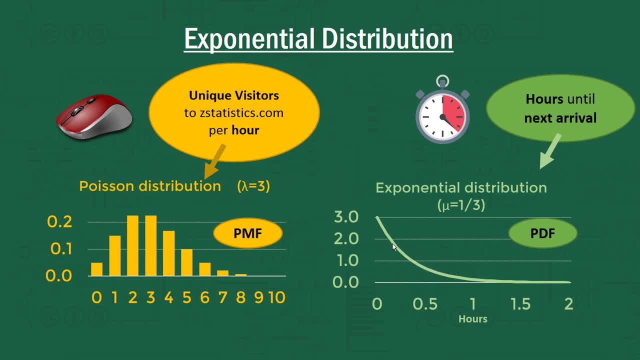 around here. It starts at the highest point and then it just keeps going down, and down and down. Why does that happen? Well, again, we'll get to that at the end of the video, So we'll first get a sense of how to use this. 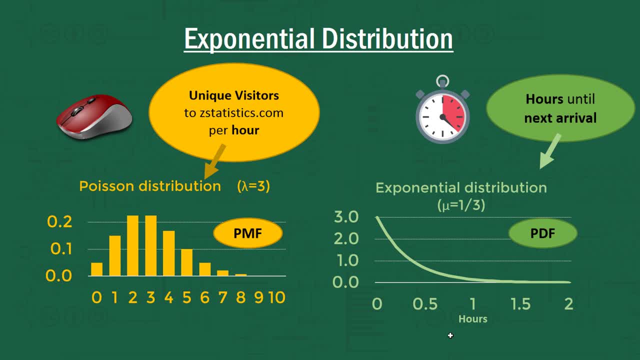 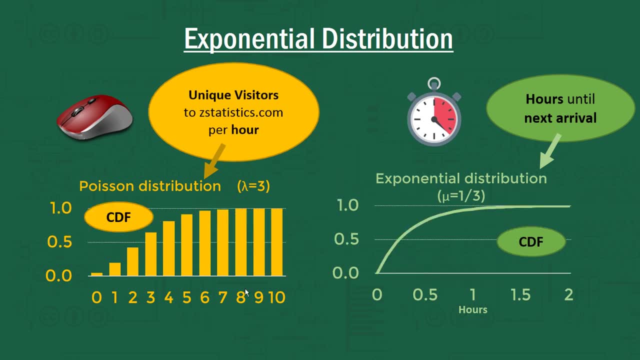 exponential distribution, And then at the end we'll deal with all that nitty gritty stuff which is really quite fascinating. So let's keep going For completion. here I've put the cumulative functions, So you can see here that the scales on the left go. 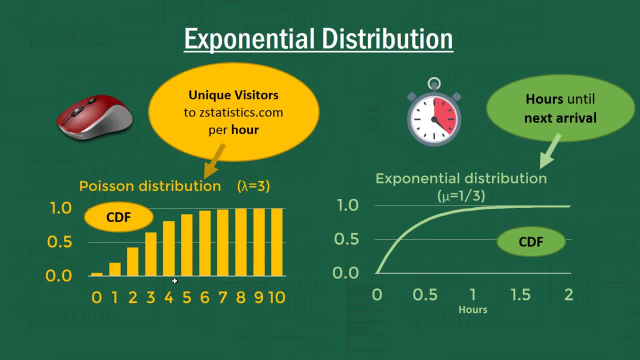 from zero to one, meaning that this represents the probability of getting, say, five and below, or six and below, unique visitors to my website In an hour. So eventually, as we start increasing this- six, seven, eight, nine, 10, it starts. 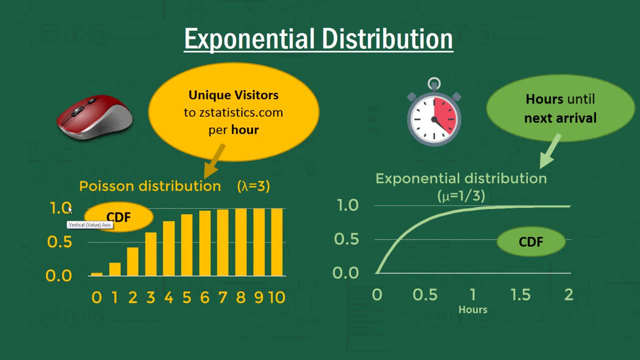 getting closer and closer to a hundred percent or one. So, similarly, over here, the cumulative distribution function. if I was trying to say what's the probability of the next arrival happening within two hours, it's going to be very, very likely because, don't forget, 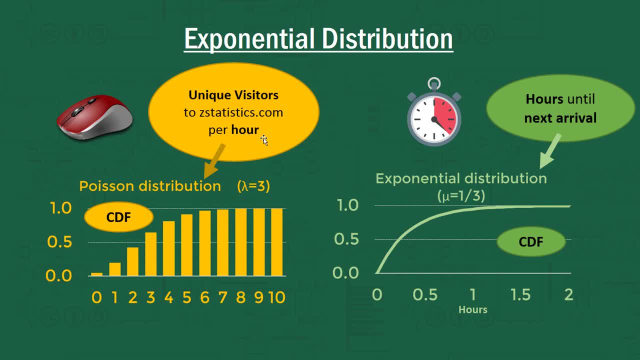 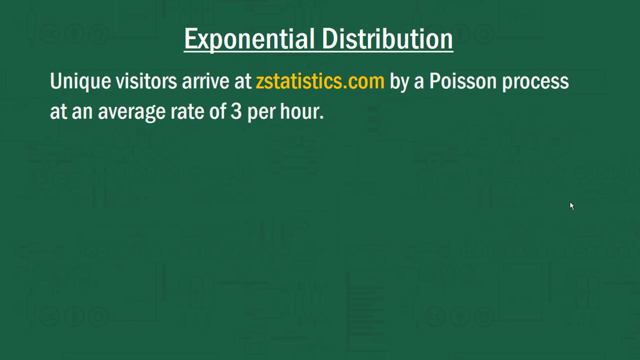 we're expecting three every hour. So the likelihood of the first arrival happening after two hours- this is very, very slim. So it's got to reach pretty much a hundred percent by two hours time. Okay, So let's actually do some calculations now. So here I've stated the question again. 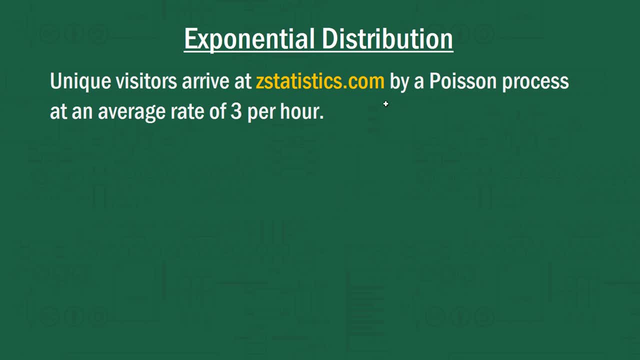 unique visitors arrive at zstatisticscom by a Poisson process at an average rate of three per hour. So I'm going to ask you to find the probability that the next visitor arrives within 10 minutes after 30 minutes passes, and then see in exactly 15 minutes. 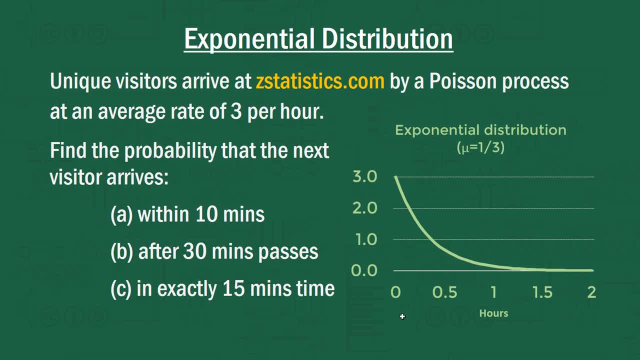 time. Now. here's that exponential distribution again, and you'll notice that we have hours here on the X axis, which is maybe not the best units for us to be using. You can say we want to probably talk in minutes here, even though that the average was given to. 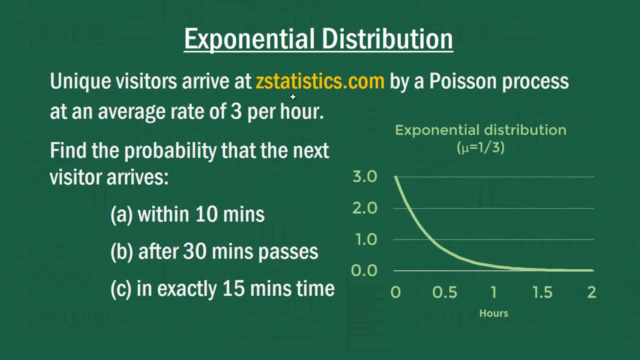 us at three per hour, right? So that would be our Poisson mean, being Lambda equaling three. So our exponential mean, Mu is equal to one on three. but the units are in hours And I do not like it. I don't like having a mean which is one on three. if I can avoid it, So let's turn it. 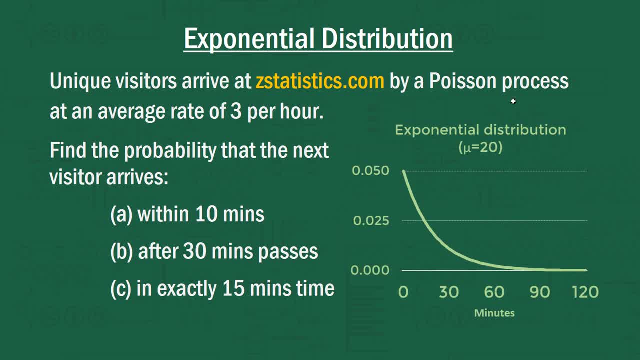 all into minutes. We know that a third of an hour is 20 minutes, right, And then the scale here goes from zero to 60 to 120 minutes, instead of zero one and two hours. So if I'm trying to find the probability that the next visitor arrives within 10 minutes, we're really 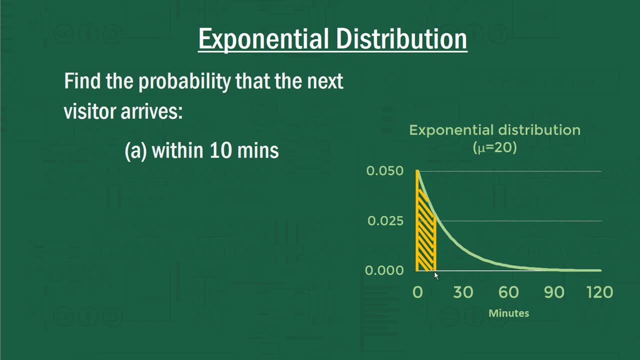 after this shaded region here, where we go from zero to about 10, imagine that's about a third of the way to 30. Right, So that shaded region is the area which represents the probability. So how do we use a formula to do this? Now, the exponential formula is provided like this: This is actually 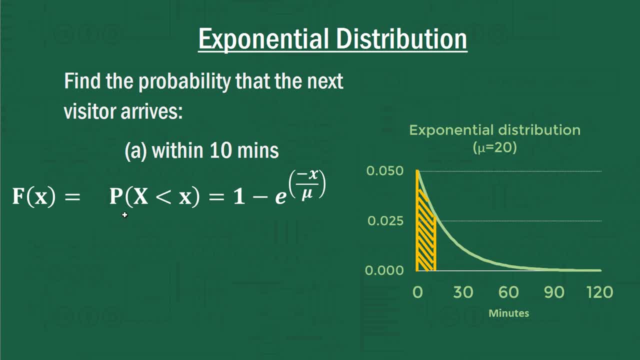 the cumulative distribution function. This provides you the probability of X, where X is the time until the next arrival, the probability of X being less than some value. So we want the probability of X being less than 10, right Now, this cumulative distribution function is provided by. 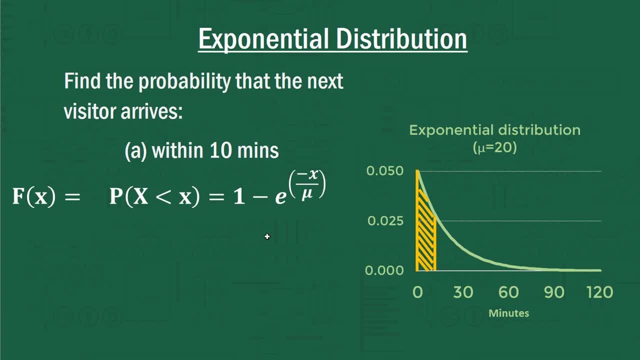 this formula here. Any statistical resource will tell you that, Although some won't provide you with mu in the formula, some will provide you with lambda in the formula And of course it will be e to the power of minus x lambda instead. 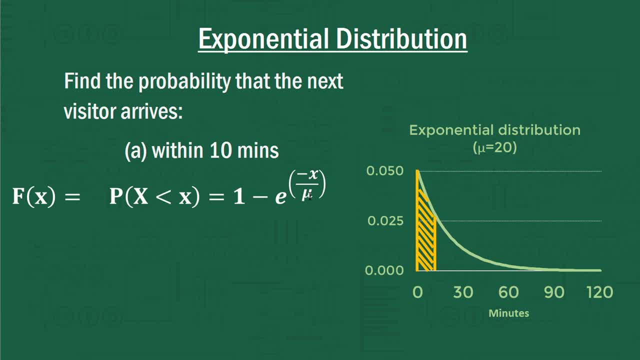 of e to the power of minus x on mu, Because, don't forget, mu is actually 1 on lambda right. So if you see a formula with lambda in it, you'll note it probably looks a little bit different, but you now know that we can get from lambda to mu. 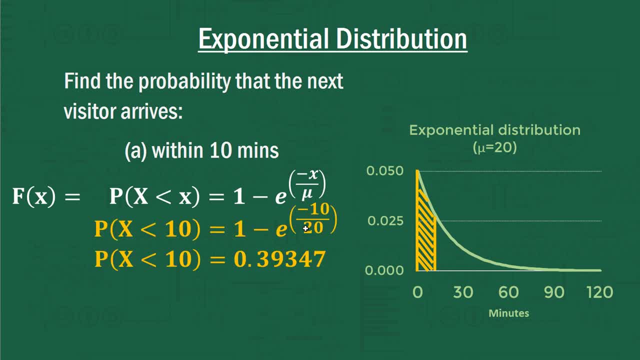 if we so need it. But I like using mu instead of lambda, because to me it makes more sense. It is the mean of the exponential distribution, which is the distribution we're using, right, Anyway, the probability of x being less than 10,. 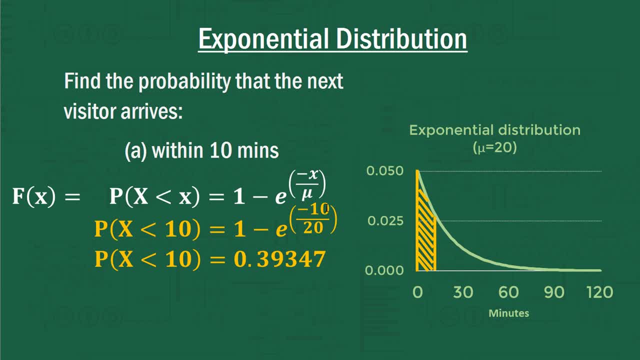 we just plug everything into the formula where x is 10,, mu is 20,, given in the question, and we get 0.39347, or 3935 is our probability. Now, that's how you would do it if you were using a calculator. But if 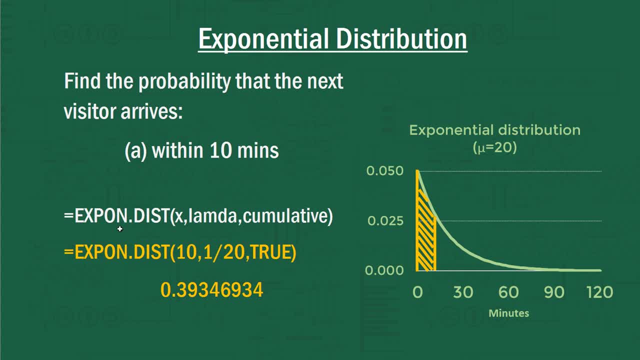 you are using Excel formula, you'll notice it has a handy exponential distribution formula. If you type the letter equals and then you write xbondist, it can actually do this calculation for you, so long as you provide it with 3.35.. 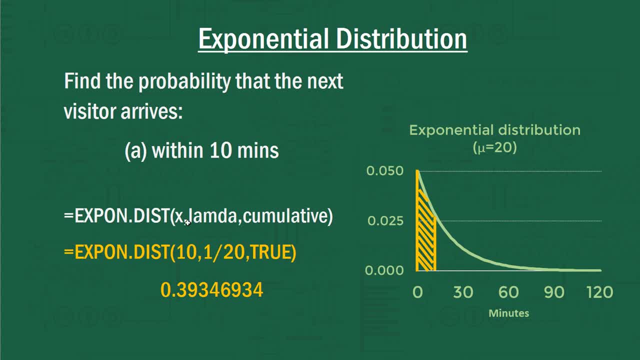 The first one is x, which is our value that we're after here 10 minutes. The next one is the value of lambda, which to me is a little bit annoying because, you know, as I said, I like dealing with the mean of the exponential distribution as opposed. 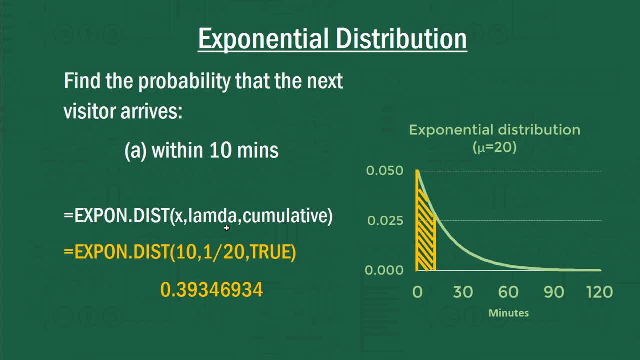 to the mean of the Poisson distribution that formed it right, Whereas the formula here it does specify lambda, which you must know is the mean of that Poisson distribution. So getting a bit confusing, isn't it? But if the mean of 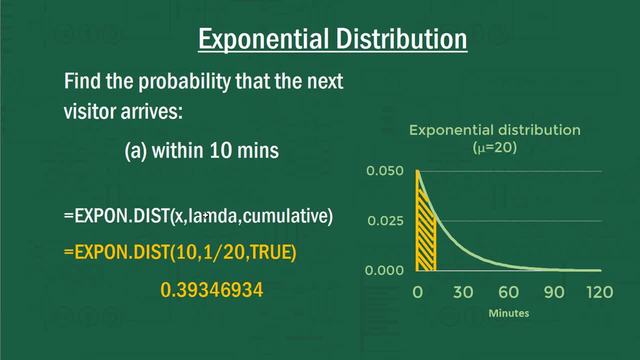 this exponential distribution is 20, the mean of the Poisson distribution is 1 on 20.. In other words, lambda has to be 1 on 20.. And then we put true, because we want the cumulative distribution up to that point. That'll give us the region below. 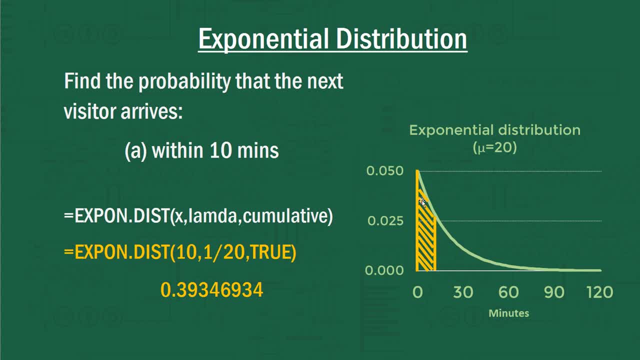 10 on the distribution. so from 0 to 10, and it'll provide us that shaded region over here And, no surprise, you get 0.39347.. Now if we're coloured in 3,, 3,, 6,, the same number we got before right. 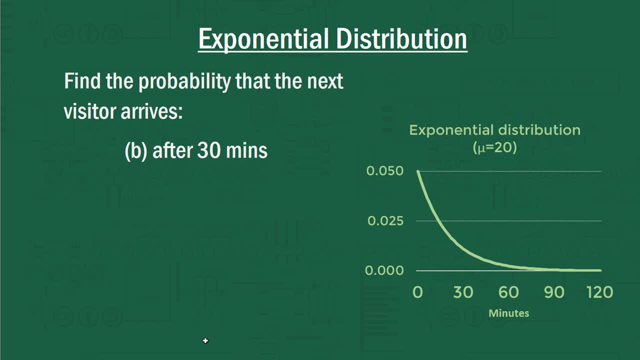 OK, let's continue, just please. OK, So let's have a look at finding the probability that the next visitor arrives after 30 minutes. So again, let's just use formula first. We can do it by hand if we want. 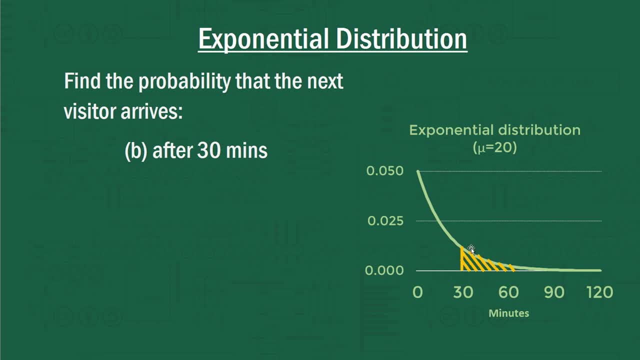 We're after the shaded region above 30 minutes. This would be the probability of the next click on my website happening after 30 minutes. So again we've got the same formula, which is the probability of x being less than 30 isjuk. 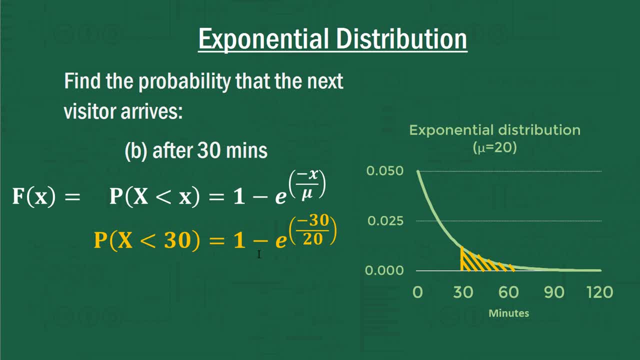 this, But of course, that's not what I'm after. I'm after the probability that x is greater than 30. So I actually need to do 1 minus all of this. Okay, so it's basically going to be 1 minus 1. 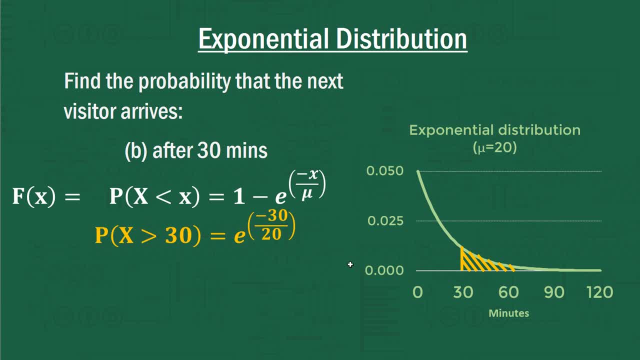 minus e to the blah blah right. That should be easy enough for you to figure out that the probability of x being greater than 30 is just e to the minus 30 on 20.. Why do we subtract it from 1?? Well, think about it. We know that this yellow shaded region has to be 1 minus the area to the 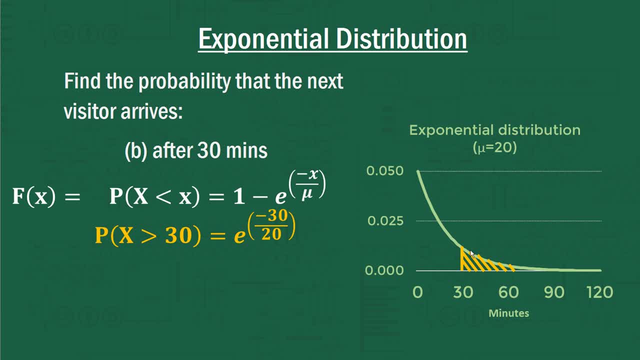 left of 30, right, Because this is a probability distribution, So the area under the curve must be equal to 1.. Anyway, so the probability of x being greater than 30 is that which, if you use your calculator, you get 0.2231,, which is great. So there's a 22.3% probability that the next 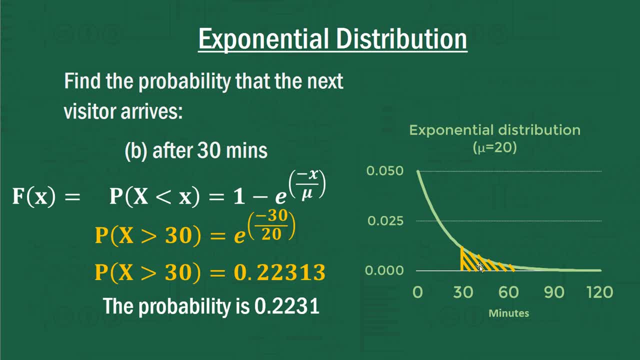 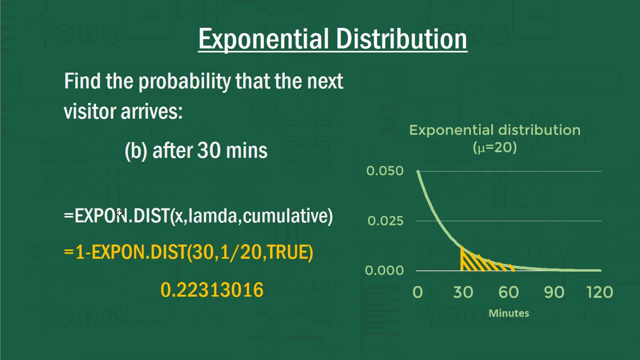 arrival on my website will happen only after 30 minutes has passed. Again, if you're going to use the formula xpondist, we have to remember that that provides us the area to the left of a particular value of x. So if we want the area to the right of a, 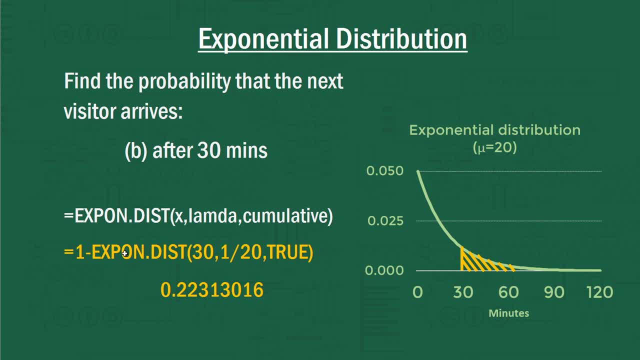 particular value of x, we're going to need to go 1 minus. So I go equals 1 minus xpondist. I put the value 30. Lambda, of course, is 1 on 20 again And I write the word true, or I can also put the. 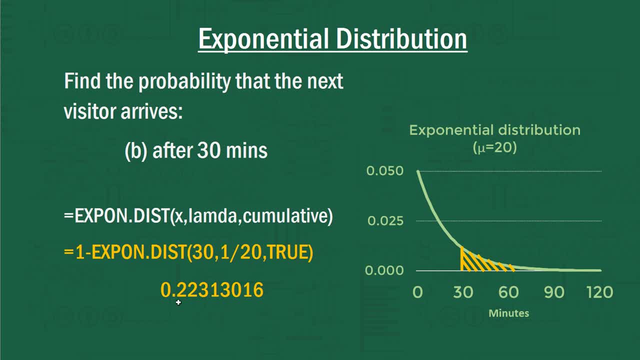 number 1 in that final argument, And that will provide me with the answer I so seek. Now, how would you answer this question? What's the probability that the next visitor arrives in exactly 15 minutes? The probability of being exactly 15 minutes is actually going to be 0.. It's essentially: what's the width of this? 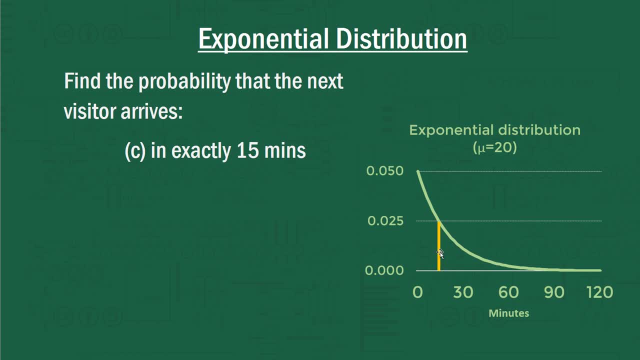 yellow line here. Now, of course, you could probably zoom in and find that this yellow line, the way I've drawn it, does have some kind of area around it, right, But it's a theoretical yellow line, right. It should have a thickness of 0,, such that the probability that x is equal to 15 is equal to 0. 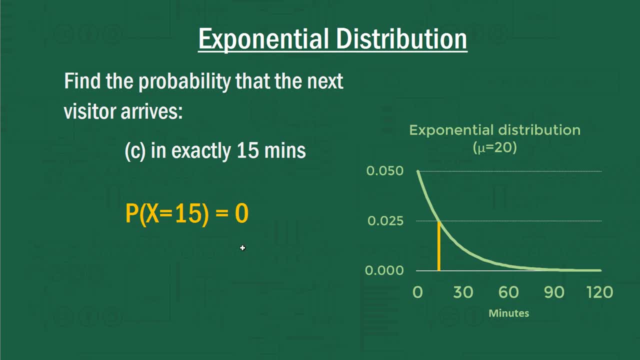 Now, if you're not quite satisfied as to how that would be, think of it this way: Can you do anything that takes exactly 15 minutes? And you might say, yeah, I can do something and then stop after 15 minutes time. That's easy, But can you Exactly 15 minutes, like 15.000000 minutes for eternity? 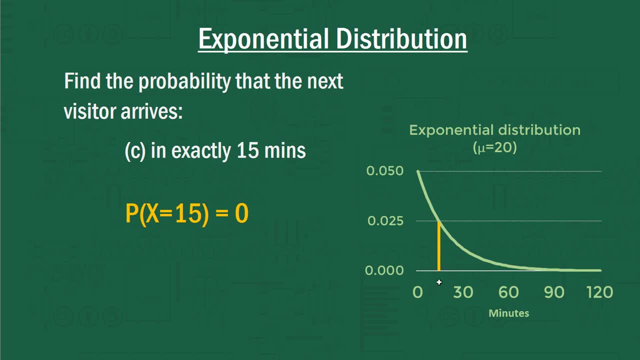 You might find that you actually can't do that, because we have a continuous distribution. We can only find the probability of being between two points, usually 0 and 15, or say 15 and infinity, But the probability of being exactly 15, as in 15.000000, is itself 0. 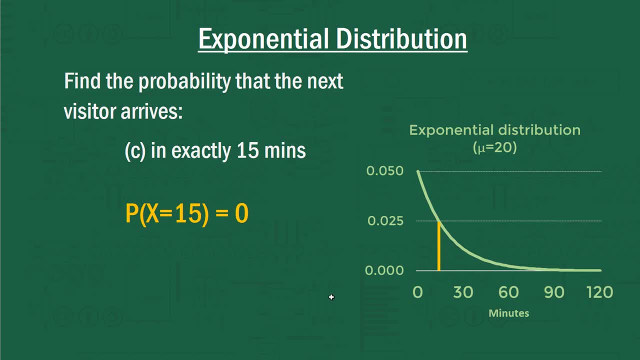 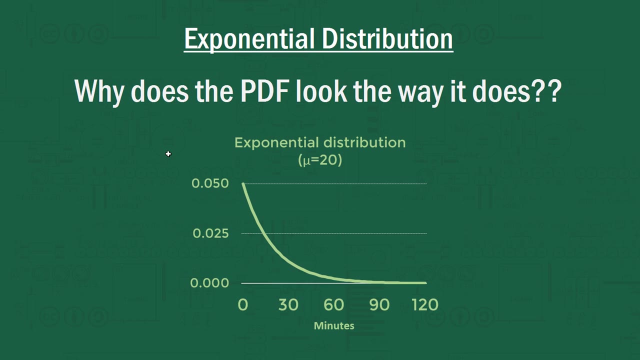 And that is the curse of the continuous distribution, Anyway. so that brings us to the end of the first part of this video, And if all you're interested in is being able to use the exponential distribution, you can kind of stop there and I've covered all the material. But if you're keen on understanding why the probability density 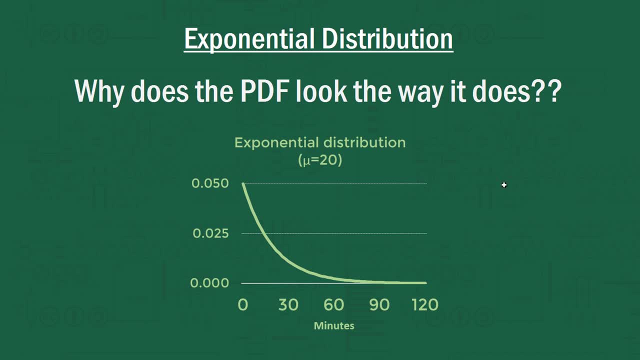 function looks the way it does, then stick with me. Let's go on a journey together, shall we? So, just to recap, we mentioned that the mean of this distribution is 20, meaning 20 minutes is the average time between visits to my website, And we've pretty much seen with most other distributions. 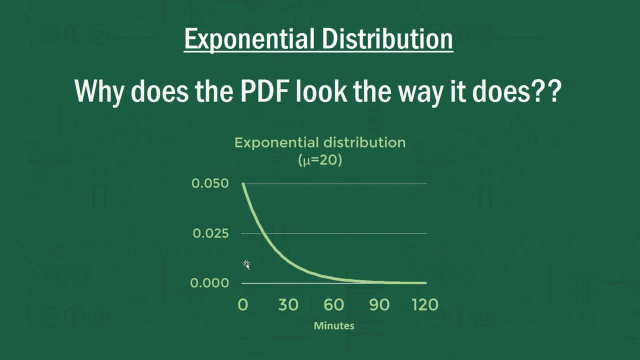 when the mean is, say, 20,, you expect a bulge at around 20, and it might trail off either side around 20.. But this doesn't really do that. It just keeps ramping downwards as we go from 0. 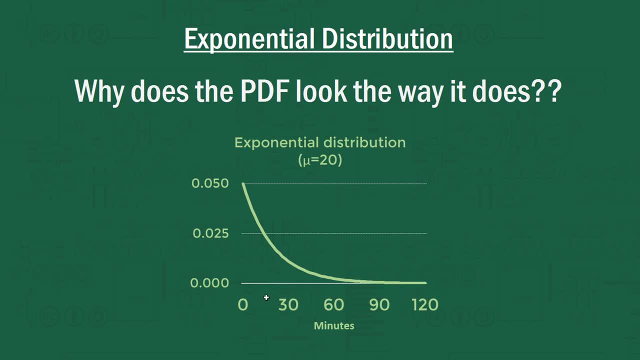 all the way to infinity. So is that suggesting that it's more probable to get a click within one minute than it is within, say, 20 minutes time? Well, not exactly. Let's open this can of worms up just a little bit. 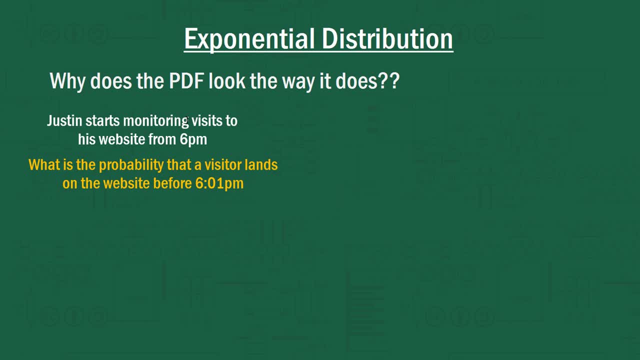 So I'll give you this example. Let's just say I start monitoring visits to my website from about 6 o'clock at night. Think about what the probability might be that a visitor lands on the website before 6.01 pm, That's within the first minute of me monitoring. Now think about this scenario. Let's just say by. 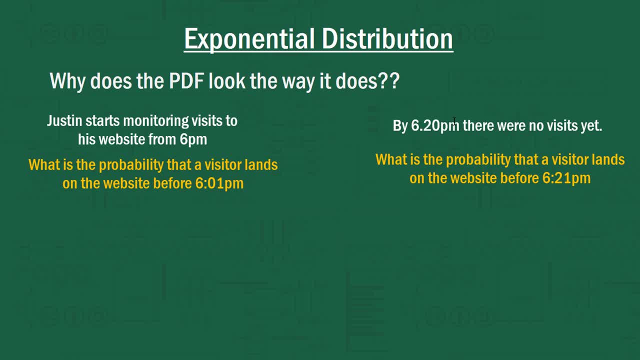 6.20 pm. I had no visits, So I waited there for 20 minutes and I got no visits within the first 20 minutes. What's the probability that the visitor then lands on the website before 6.21 pm? 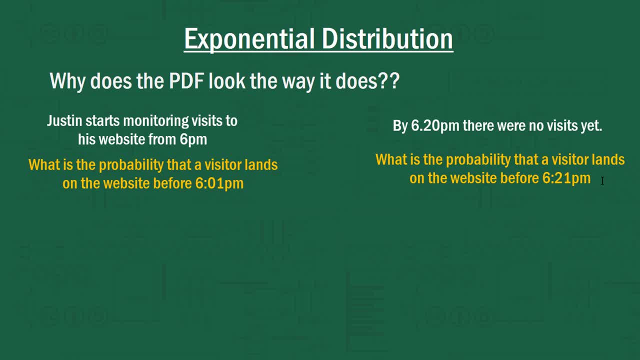 Hmm. Now, if I asked you what your gut feeling is about these two probabilities- and I might even just put a little question mark here to make it look like a question- you might start thinking that, yeah, the one on the right here is more probable. 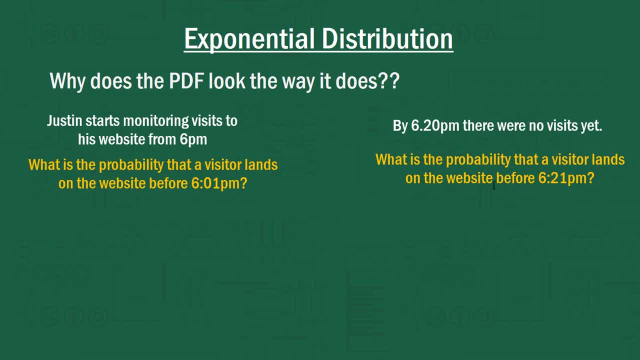 right. We've already waited 20 minutes, So it's probably more likely that someone's going to be there in the next minute on the right side here than it does on the left side. But guess what? They're actually the same probability. But guess what? They're actually the same probability. 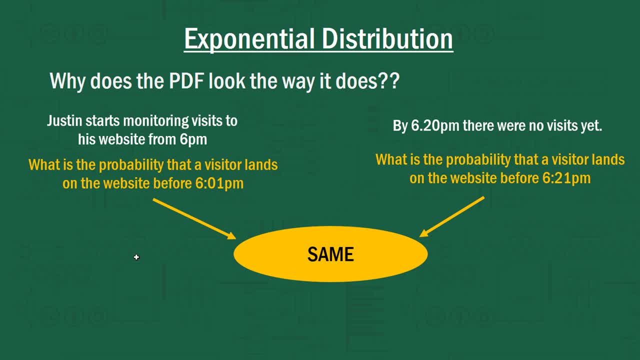 And this is due to that principle of memorylessness. The exponential distribution doesn't care that you've waited 20 minutes already with no visits. It's still that same probability in the next minute. So this is the first step to understanding why this PDF looks the way it does. This is that 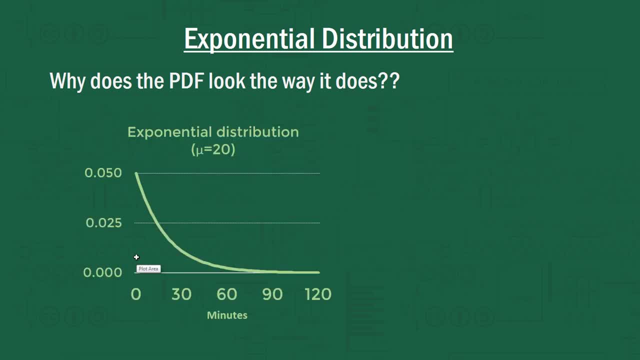 principle of memorylessness. Now here's the second bit. We'll repeat the same question: What's the probability that the first visitor lands on the website within the first minute And we can actually find an answer to this question using the formula that we were using previously? I'm not. 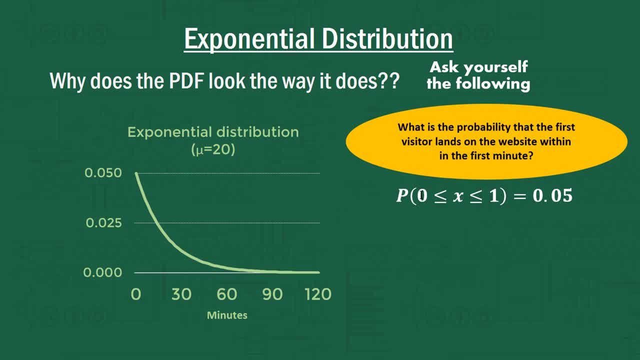 going to show you how to do it, but it turns out that the probability of X being between zero and one is about 0.05.. So there's about a 5% chance of the first visitor to my website coming within the first minute of me monitoring. So now let's have a think about what the probability might be. 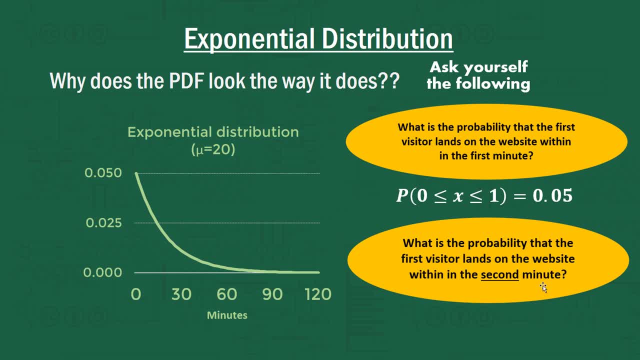 that the first visitor lands on the website within the second minute. Now, the first thing we need to understand about this second scenario here is that it's comprised of two distinct events. The first visitor must not land on the website within the first minute. 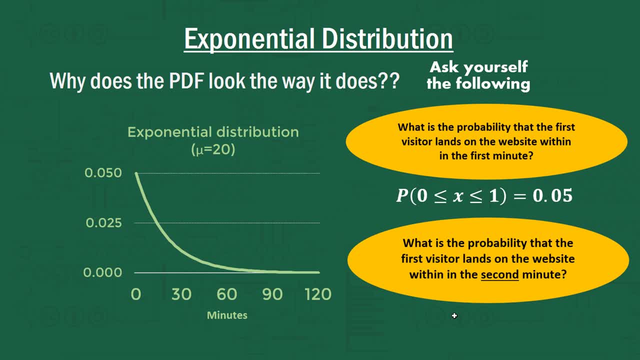 and then this visitor must land on the website within the second minute. So to find the probability that X lies between one and two, we actually have this 0.95 multiplier that comes in, So we can see that the first visitor lands on the website within the first minute. 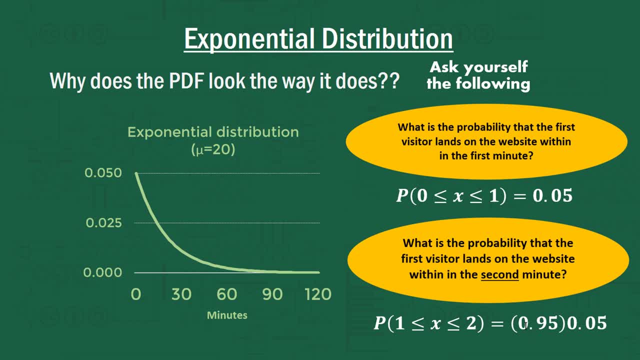 and then the second visitor lands on the website within the second minute. Why do we multiply by 0.95?? Well, as I said, the first thing that needs to happen for this to be true is that the first visitor can't arrive within the first minute, And the probability of that is. 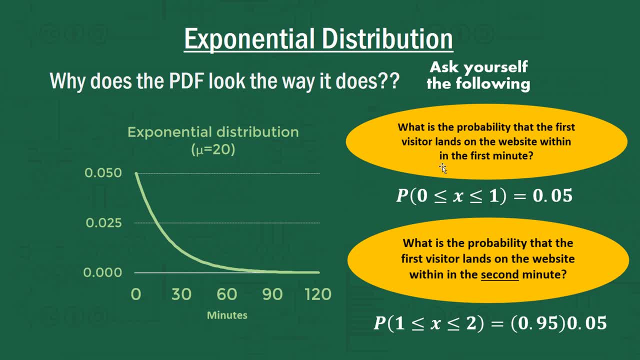 one minus 0.05, which is 0.95.. So we already know that we have this 0.95 multiplier going on, And then the next thing that needs to happen is that this first visitor needs to arrive within the next minute, and we already know what that probability is: It's 0.05,. 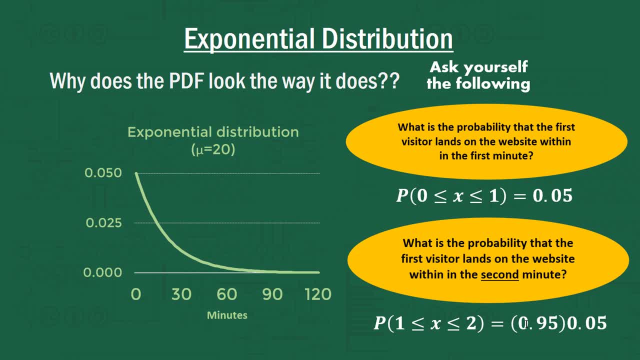 thanks to the memorylessness of the exponential distribution. All right, so let's see what happens now when we move this along to the third minute. So if I'm asking what the probability is that the first visitor lands on the website within the third minute, in other words, between two and three minutes, you can see that we're going to have two. 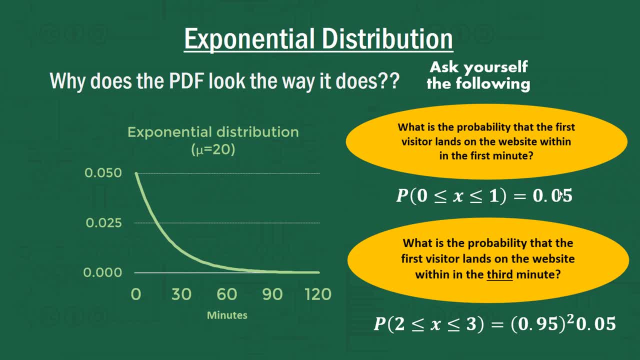 of these 0.95.. 0.95 multipliers come in because not only did this first visitor need to miss the first minute, so 0.95, it also needed to miss the second minute, which is another 0.95. and finally,